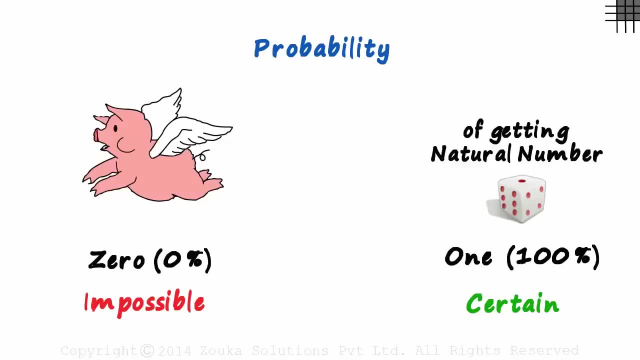 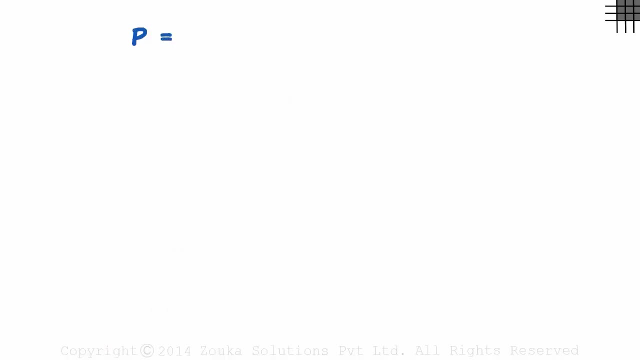 That brings us to an important point in the video. The probability of every event will lie between zero and one inclusive. But how is it actually defined? What is probability? Let's call it P. The probability of an event occurring is the number of ways in which an event can occur. 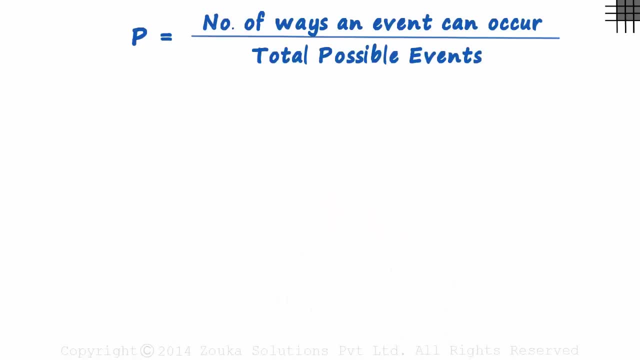 over the total number of possible events. Number of ways an event can occur over the total number of events. To understand this well, we look at three examples. First, the toss of a fair coin. It can either land a head or a tail. 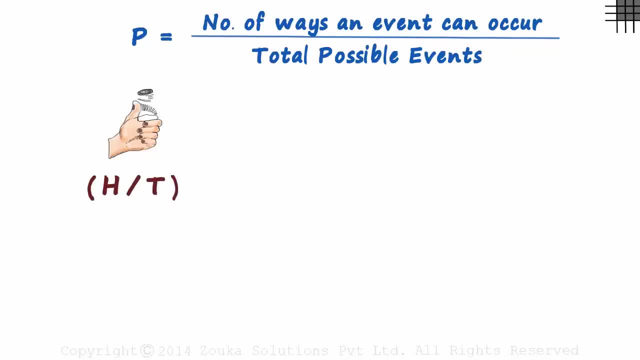 Now listen to this carefully. If we toss a fair coin, what is the probability that it will land a head? We are just tossing one coin. What is the probability that we will get a head? What is the number of ways in which we can get a head? 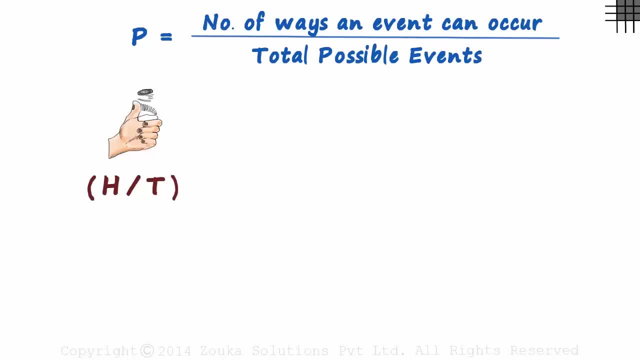 There's only one way, and that's if it lands a head. And what are the total possible events? We can get a head or a tail, Two total events. So the probability of getting a head at the toss of one fair coin is one over two. 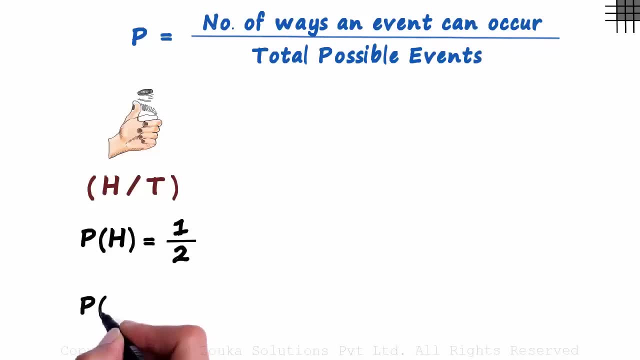 or fifty per cent. What is the probability of getting a tail then? There's only one way in which we can get a tail And there are two possibilities. Probability of getting a tail at the toss of a coin is also fifty per cent. 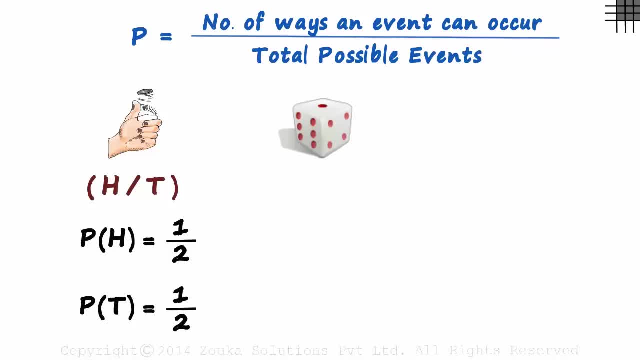 Now let's look at the case of a fair die. If we roll a fair die, it will land one of these six numbers. What is the probability that the die will land a three? This one's easy. There's only one way in which we can get a three. 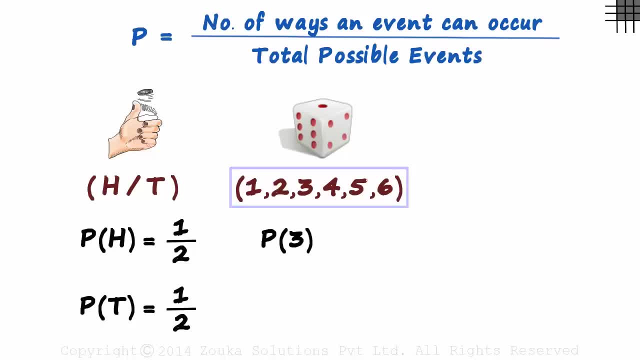 And there are a total of six possibilities. The probability of getting a three at the roll of a die is one over six. It's slightly on the lower side, Okay. so what would be the probability of getting an odd number at the throw of a fair die? 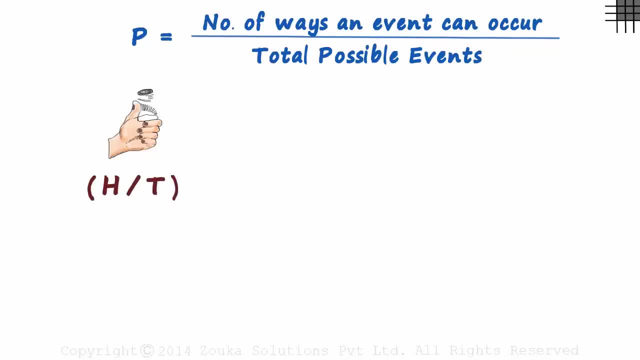 Now listen to this carefully. If we toss a fair coin, what is the probability that it will land a head? We are just tossing one coin. What is the probability that we will get a head? What is the number of ways in which we can get a head? 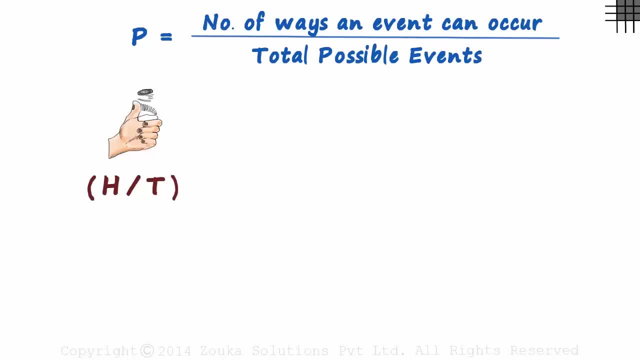 There's only one way, and that's if it lands a head. And what are the total possible events? We can get a head or a tail, Two total events. So the probability of getting a head at the toss of one fair coin is one over two. 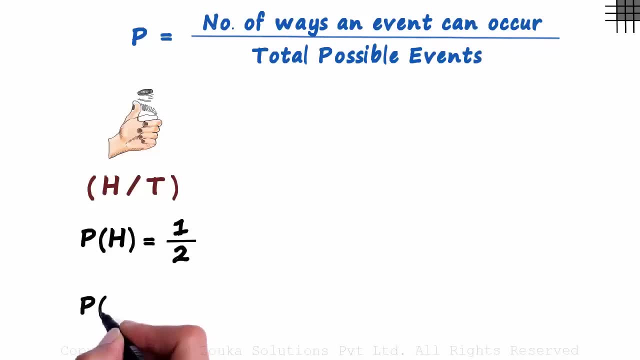 or fifty per cent. What is the probability of getting a tail then? There's only one way in which we can get a tail And there are two possibilities. Probability of getting a tail at the toss of a coin is also fifty per cent. 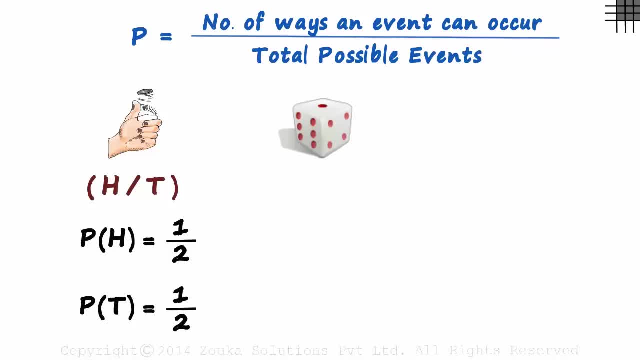 Now let's look at the case of a fair die. If we roll a fair die, it will land one of these six numbers. What is the probability that the die will land a three? This one's easy. There's only one way in which we can get a three. 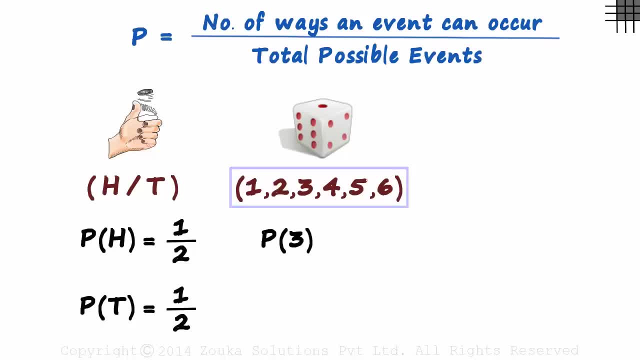 And there are a total of six possibilities. The probability of getting a three at the roll of a die is one over six. It's slightly on the lower side, Okay. so what would be the probability of getting an odd number at the throw of a fair die? 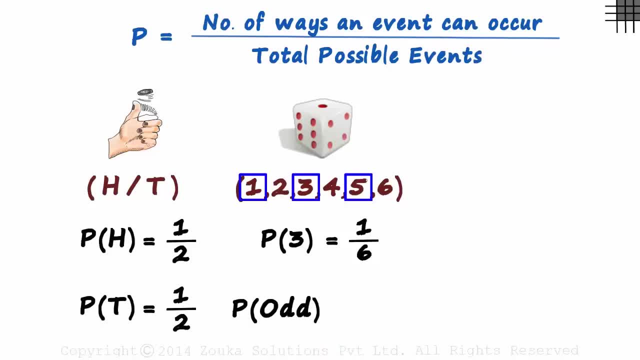 There are three ways in which we can get an odd number, And there are a total of six possibilities. So the probability of getting an odd number at the throw of a fair die is three over six or fifty per cent. And the last example is that of a pack of cards. 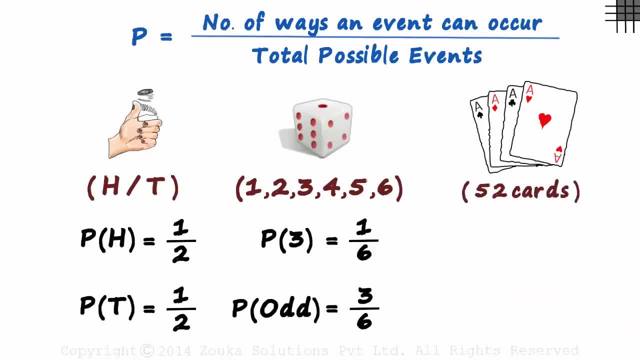 Let's assume a pack of fifty-two cards. Say we pick a random card from this pack, What is the probability that we will pick a jack? Think logically: How many jacks are there in the entire pack? There are four jacks. 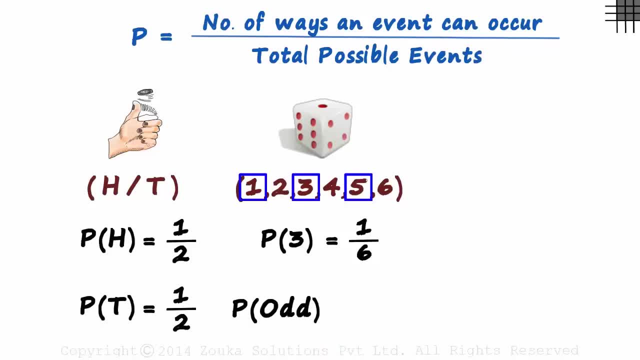 There are three ways in which we can get an odd number, And there are a total of six possibilities. So the probability of getting an odd number at the throw of a fair die is three over six or fifty per cent. And the last example is that of a pack of cards. 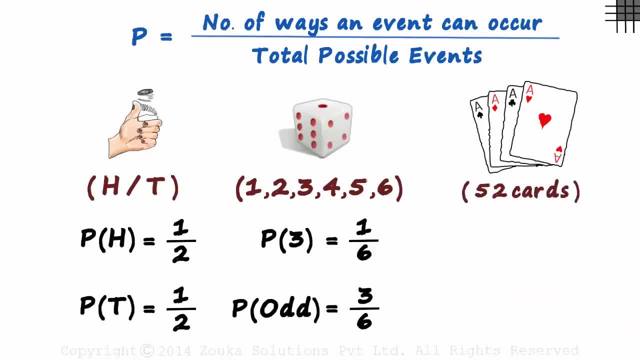 Let's assume a pack of fifty-two cards. Say we pick a random card from this pack, What is the probability that we will pick a jack? Think logically: How many jacks are there in the entire pack? There are four jacks. 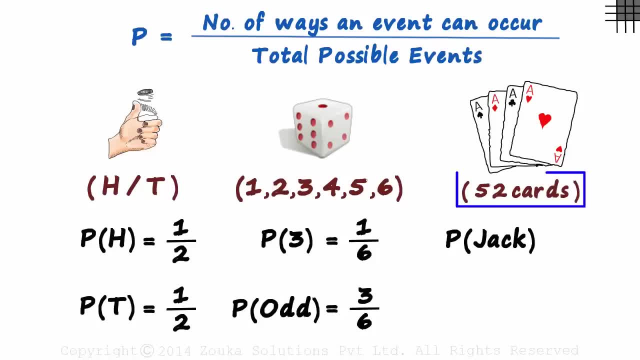 One in each suit And the total number of cards is fifty-two. The probability of picking a jack from a pack of fifty-two cards is four over fifty-two. And here's the last question in this session. What is the probability of picking a face card? 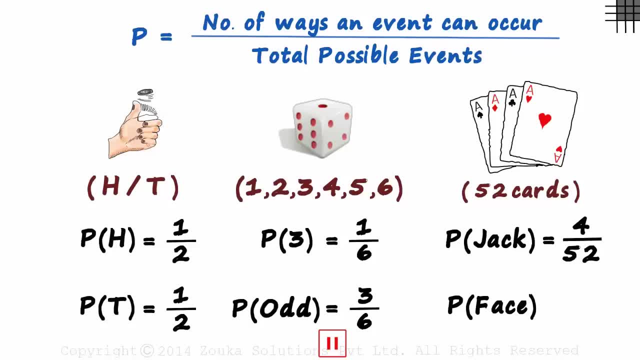 What is the probability of picking a face card from a pack of fifty-two cards? There are twelve face cards- Jack, queen and king- in each of the four suits And the total number of possibilities is fifty-two. The probability of picking a face card from a pack of fifty-two cards is twelve over fifty-two. 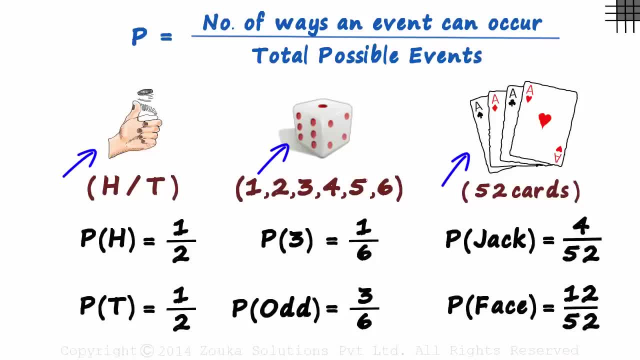 These are the three most common types of problems seen in the exams. In the coming sessions we will solve more problems based on these three examples.